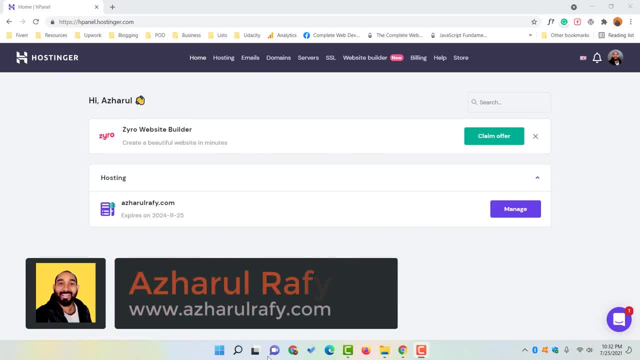 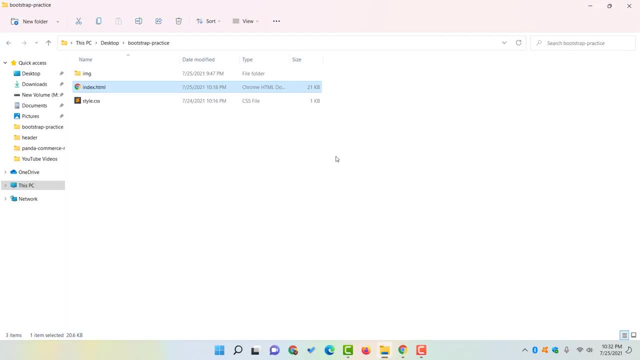 Hello and welcome back. This is Ishkul Rafi once again. From this video you are going to learn how to host a custom coded website on Hostinger hosting plan. So first of all, let me show you the website data which I have got here. As you can see, I have got indexhtml, stylecss and. 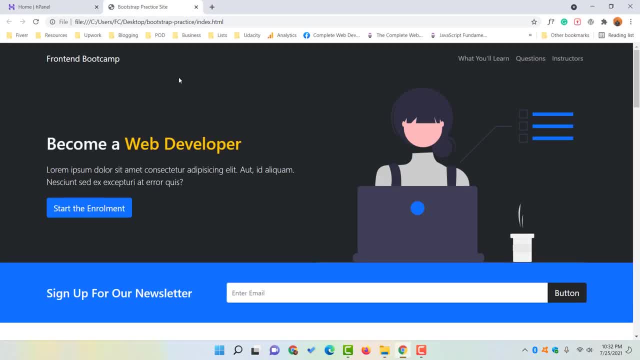 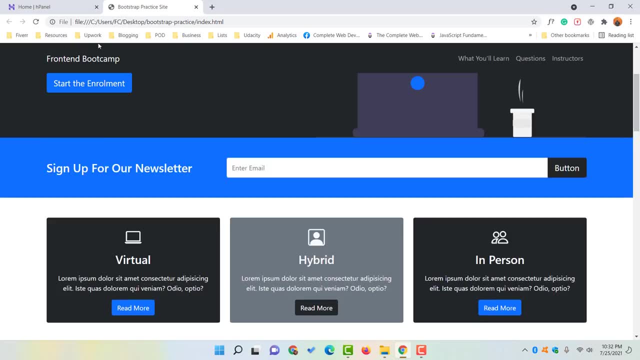 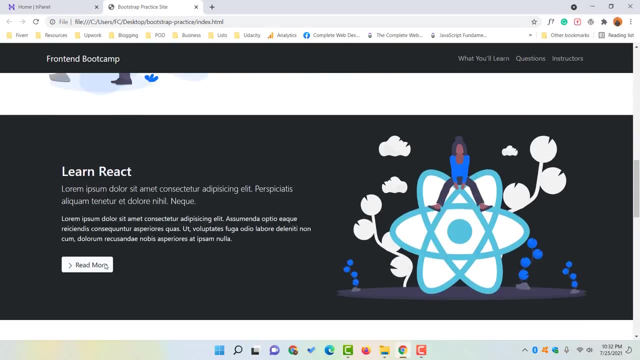 image files for the website. So let me open this website, and you are going to see. this website is being opened in our Chrome browser. But only problem is, as it is hosted on my local computer on C drive, I am the only person who is being able to access this site. But now I want to host. 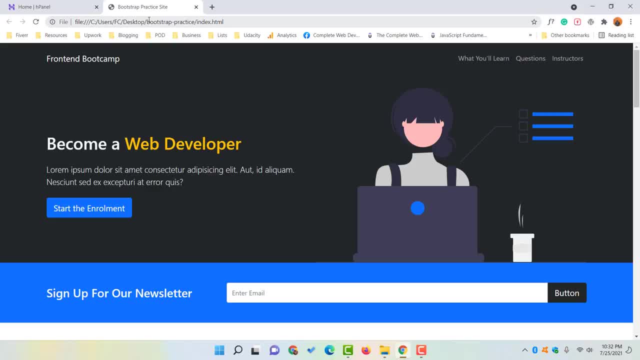 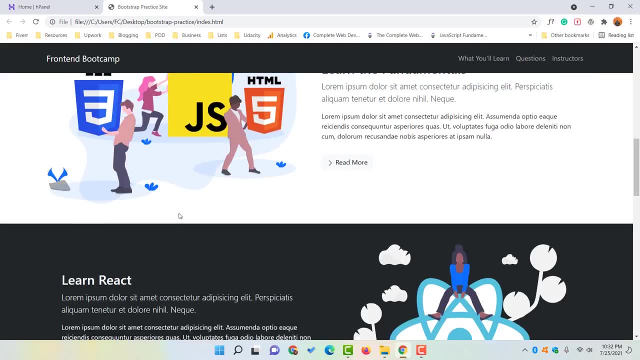 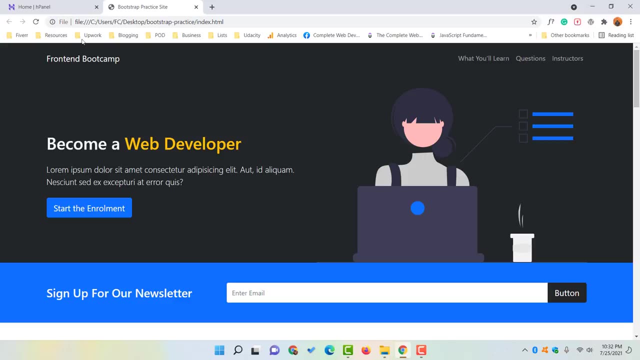 this website on a domain and hosting plan, so that anyone will be able to access by that domain name and will be able to view all the contents inside this website. So let me show you the step by step process on how we can host our custom coded website on Hostinger hosting plan. So let me 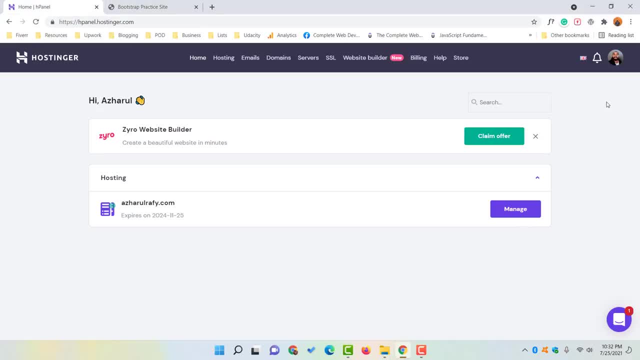 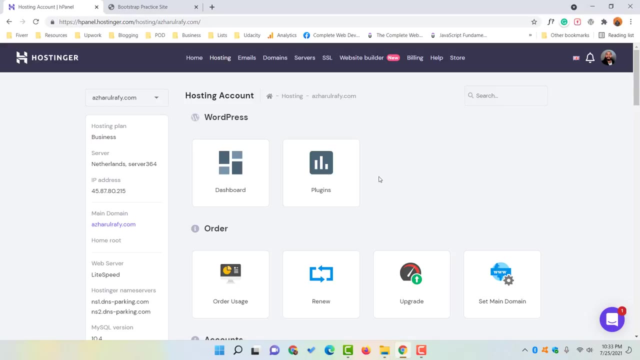 take you to my Hostinger hosting account. After signing in, you are going to see your hosting plan here. Simply you have to click here on this name, or you can click on this manage button right here as well, which is going to take you to your control panel of the hosting. And after coming up here on 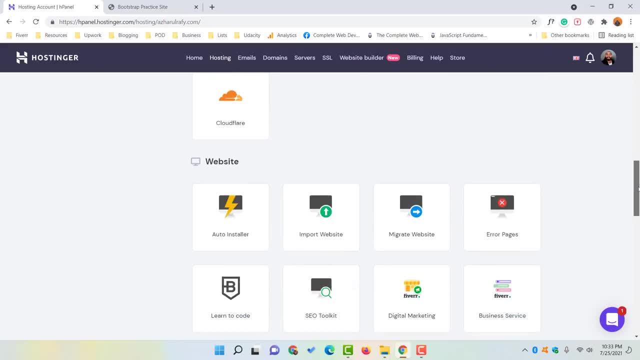 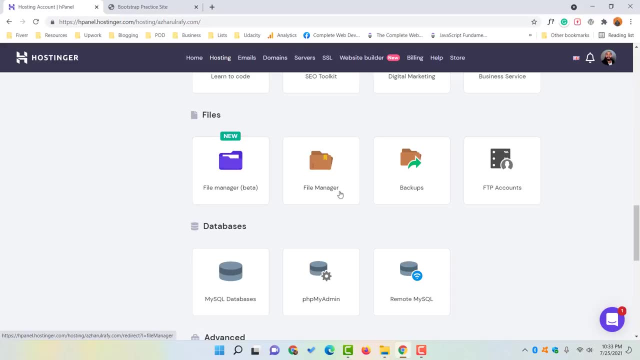 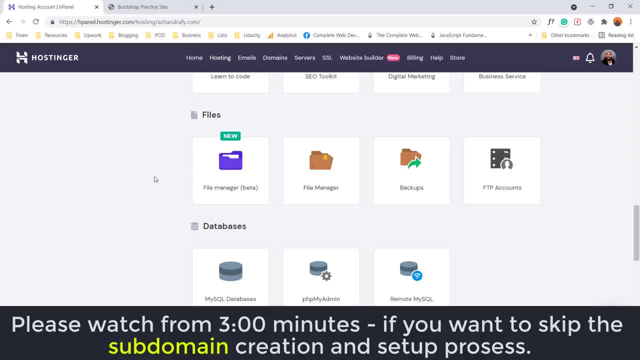 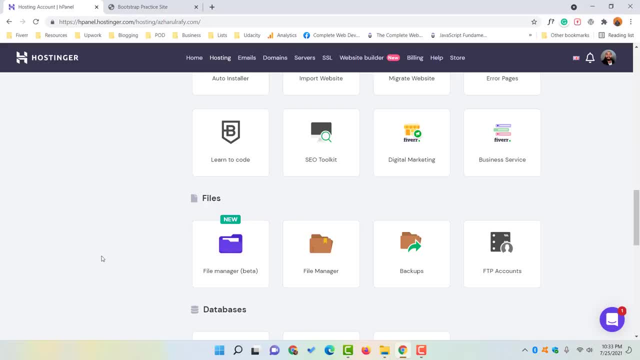 hosting plan, So let me take you to my Hostinger. hosting plan- So let me take you to my Hostinger. i would love to create a sub domain so that the website will be hosted on a sub domain and then we can continue to the process of hosting the site. right? so to create a sub domain, i have to go a. 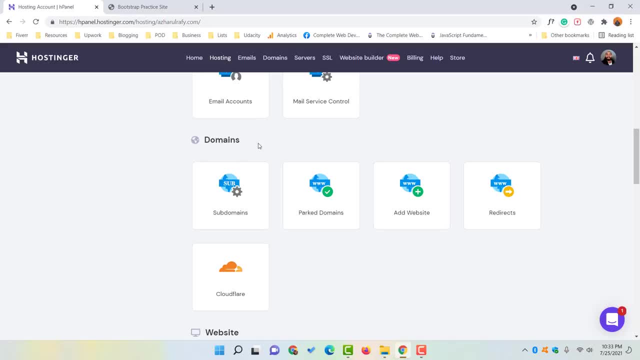 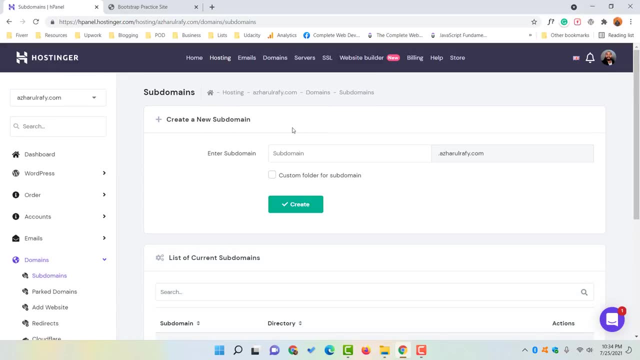 little bit up until i find this domains option and from this sub domains- so let me click on this sub domains- we'll be able to get this option to create a new sub domain under this domain name, which is astrographycom. so let me create the sub domain. let's say, boots, drop one dot as photographycom. 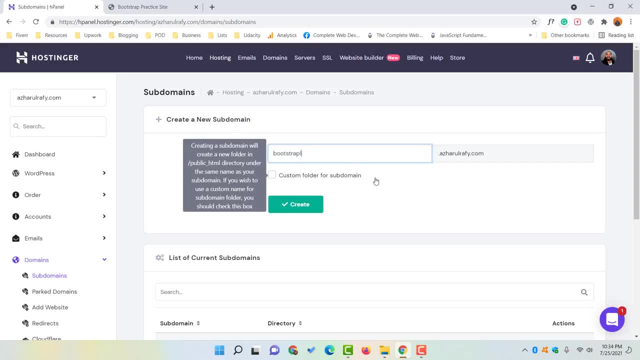 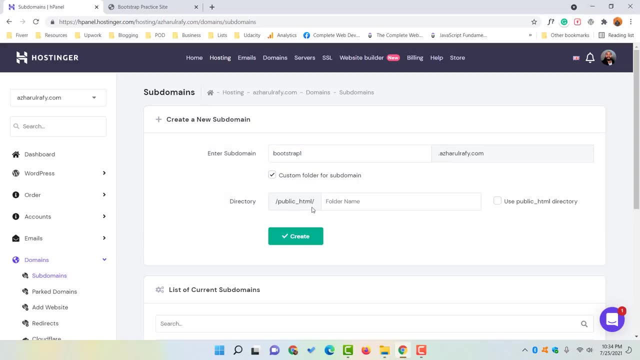 after that, i would love to host this website on a custom directory or custom folder. so let me click on custom folder for sub domain. after that, it is going to be placed inside public html. after that, the name of the folder is going to be, let's say this: one bootstrap, one right, and after that. 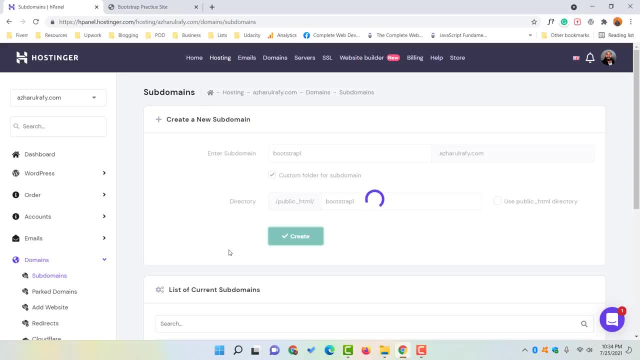 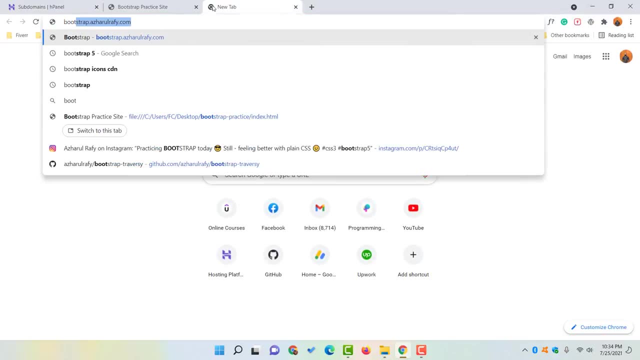 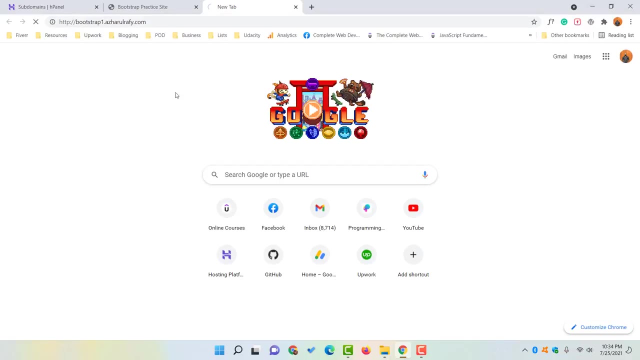 i have to click on this create button right here and the sub domain is going to be created successfully. just take a look. so now, if i visit, let's say, b, double, o, t, s, t, r, a, p, one dot as harold rafi dot com, you are going to see, nothing is going to be appearing here. instead of this, let's say: 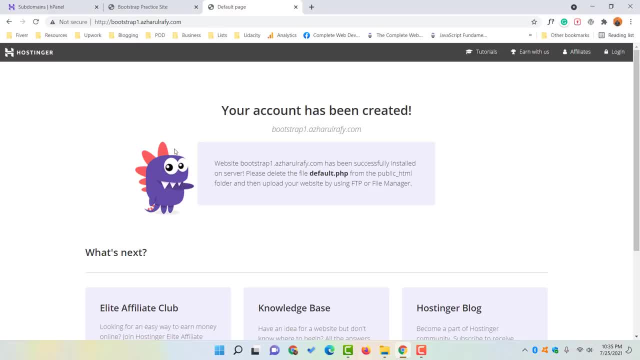 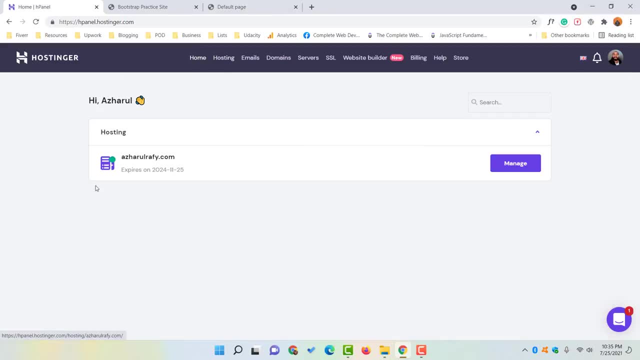 this default page. so we are done with the domain setup. now it's time to go back to our cpanel, and then let me take you directly to our cpanel. and then let me take you directly to our cpanel, and then let me take you directly to the home page. we can actually go from there as well, and after 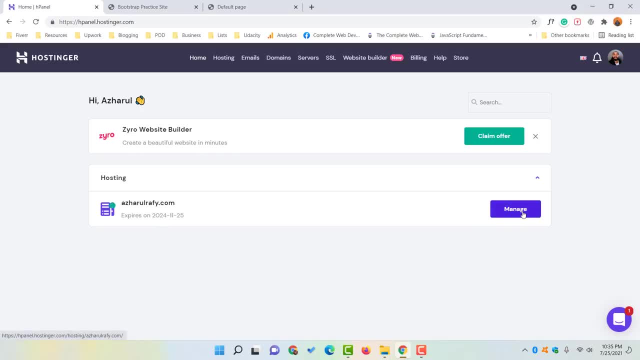 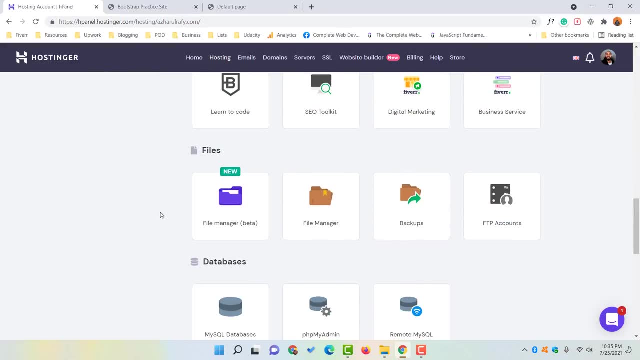 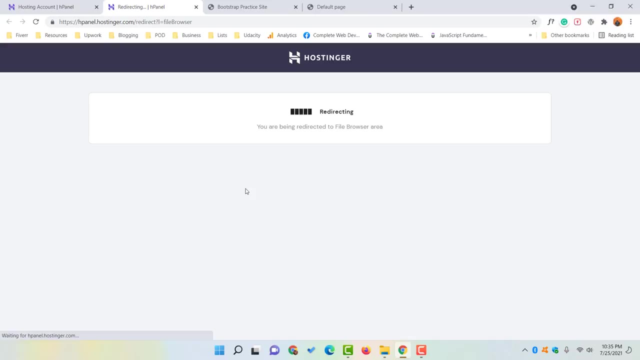 coming up to the home page, we have to go again, click on manage, after that go a little bit down until we find, let's say, this files option and let me use this file manager option. so let me click on file manager and it is going to take us to the file manager folder of our hosting plan, where 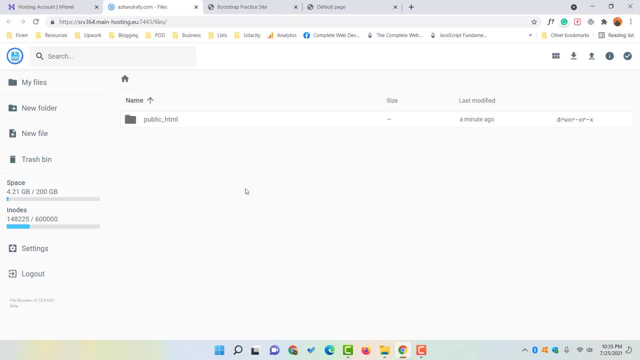 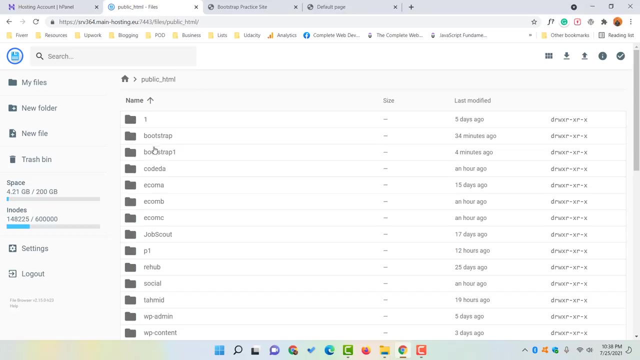 we'll be able to see all the domains that we have hosted under this hosting plan. so let me click on public html and, as i have already mentioned, the folder we have just created is going to be inside this public html, so let me double click and now we are going to see all the other folders. 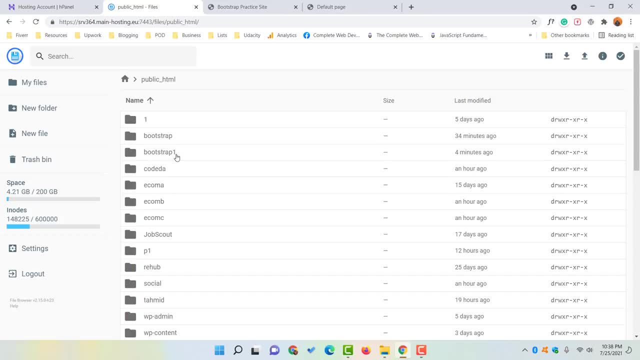 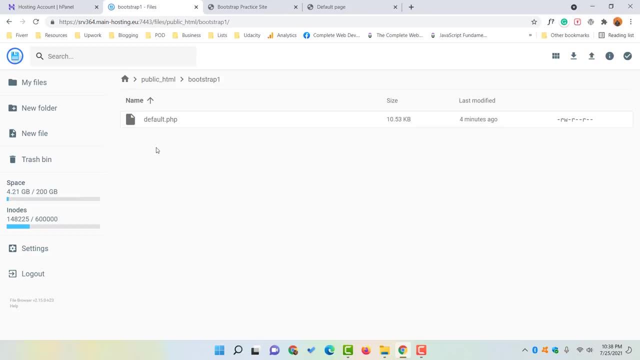 which we created previously. so, as you can see, here is the folder which we have created. so now i have to click on this bootstrap one and after that, simply, you are going to find this option: default dot. php. now what we have to do? we have to click on. 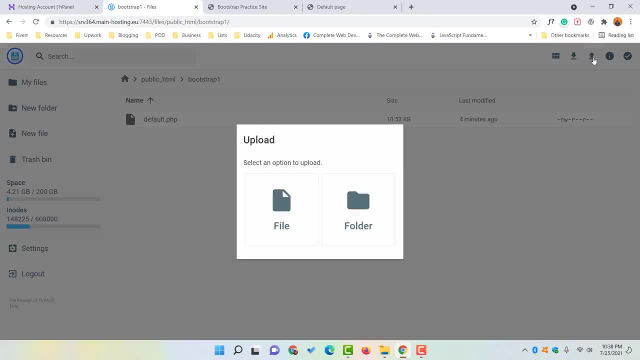 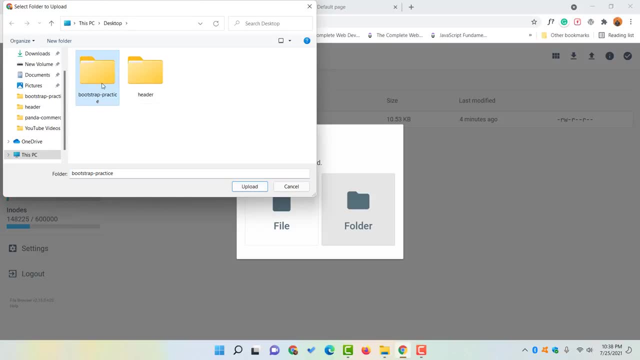 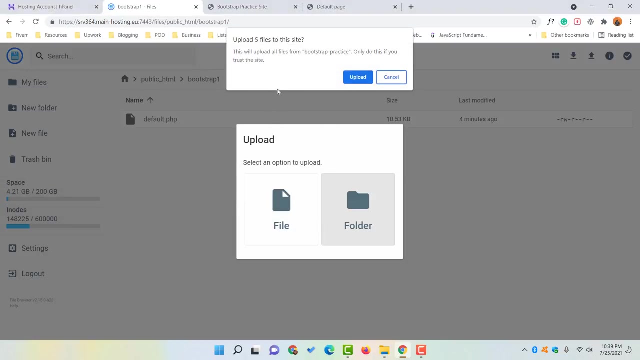 to simply click on this upload icon right here. after that, let me click on this folder, and then we have to select the folder which we have to upload. so this is the folder which is containing our website contents, so let me select. after that, let me click on upload. it is going to show you. 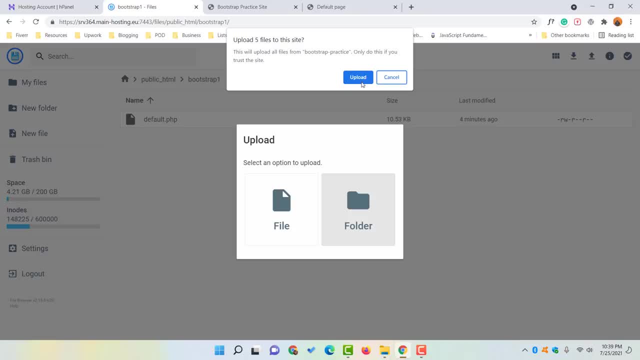 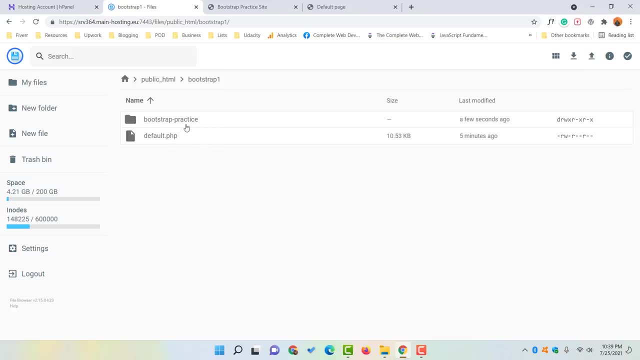 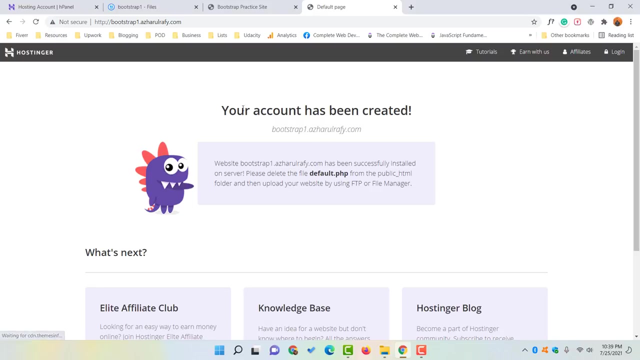 this warning message: upload five files to this site. so let me click on upload again and here we go. the website, or the data has been uploaded. now if we visit this website again, as you can see here, bootstrap1.ajaruraficom, you are going to see this exact page. the reason is because 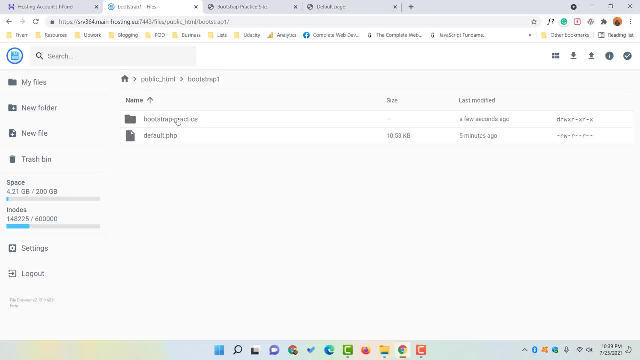 we have to move the folder. sorry, move the files from this folder to this folder in this place, right? so let me take you inside this bootstrap practice folder. after that we have to select all of these items. so i have selected image. now i'm going to shift. click on shift in my keyboard, then click here. 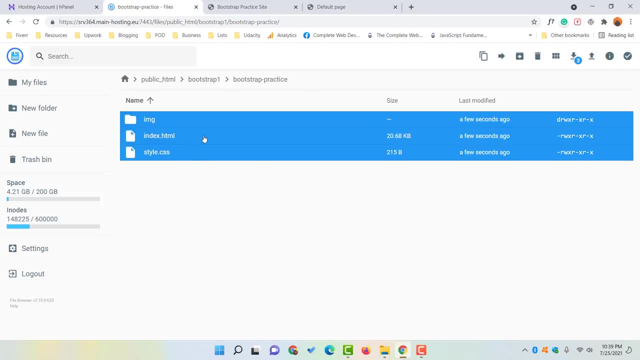 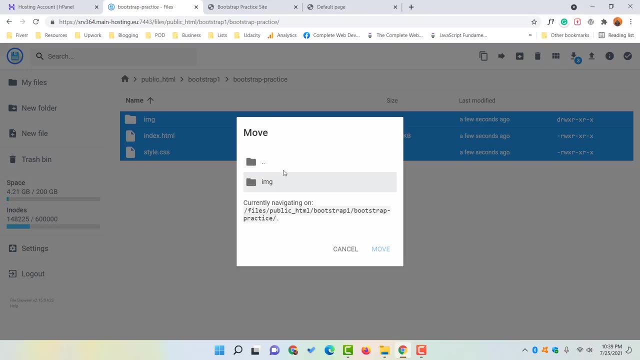 so that all of these files will be selected. then click on the right button of your mouse, then click on move file. after that i have to click double time or two times here. it is going to take us outside of this folder. then again, double click here and you are going to see this folder, right. 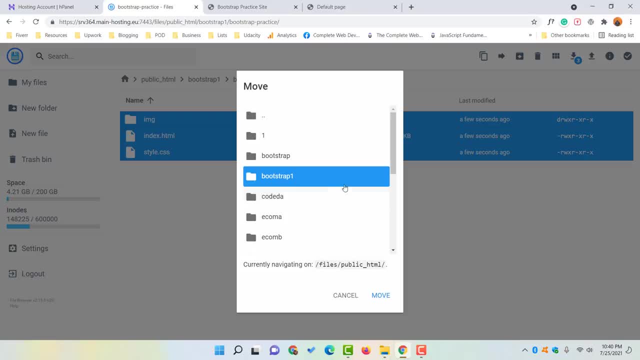 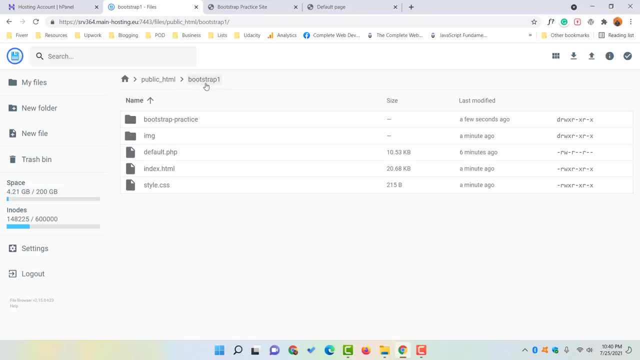 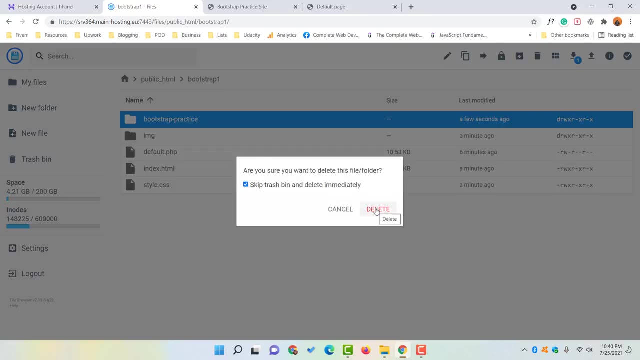 so bootstrap one. so let's select the folder. after that we have to move the file to this folder, and here we go. the website also has been uploaded. that click on move and the files are now inside this bootstrap one folder. right, so now we can simply delete this file from here or this folder, and we can also delete this default dot PHP file. 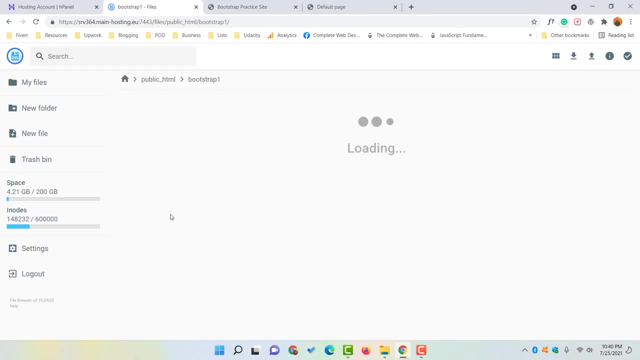 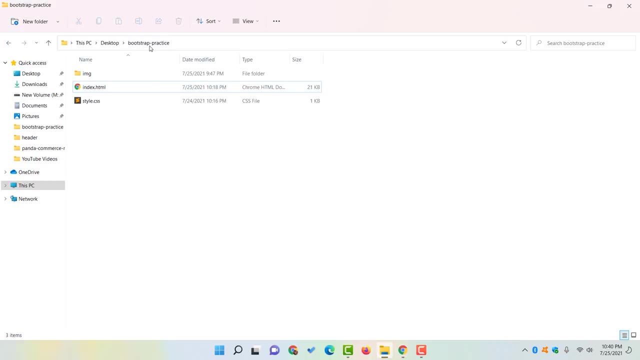 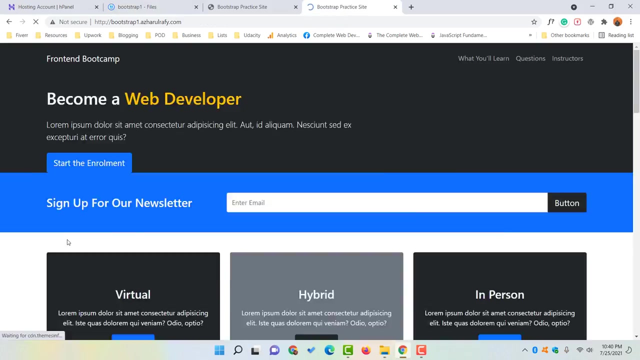 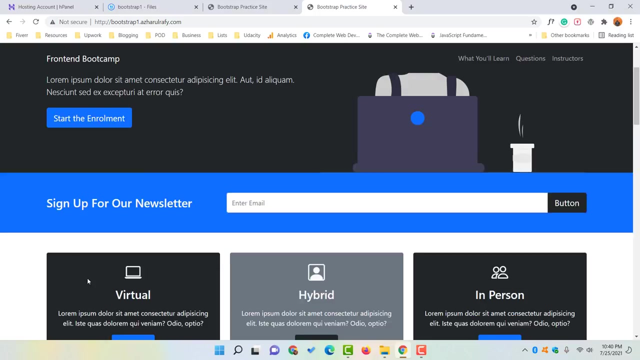 as well. all right, so now we have got only the data, or only the contents which we had on our folder, right on our computer. now let me take you back here. after that, if I reload this page, you are going to see our website is working perfectly fine, right? so this was the process of how to 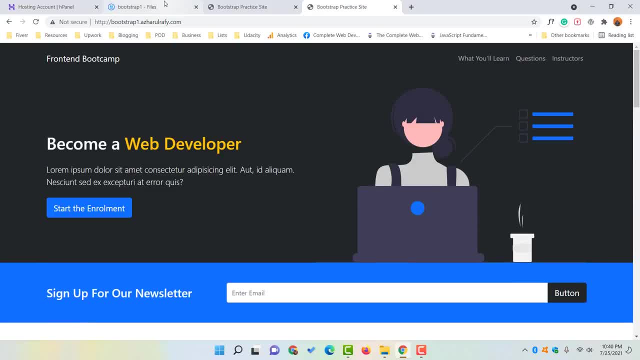 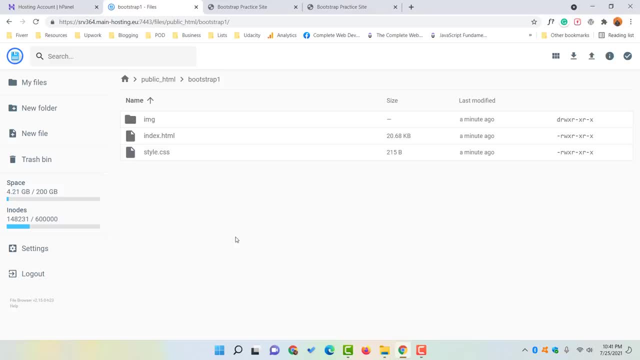 upload a custom-coded website on Hostinger hosting plan and I believe you have found this video helpful. if you did, please give this video a like, share this video to help your friends and please don't hesitate to ask me if you have any questions. please do not hesitate to ask me if you have any.